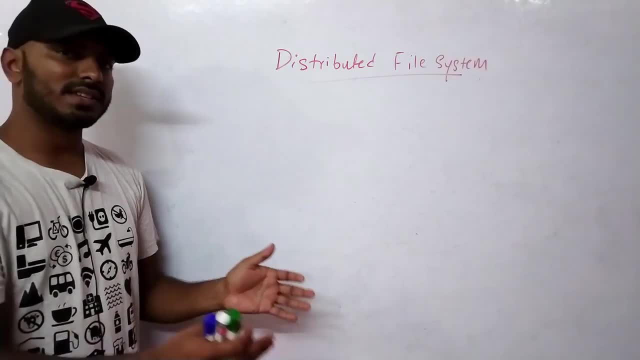 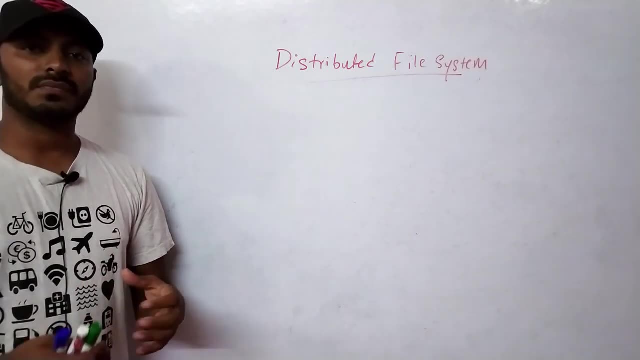 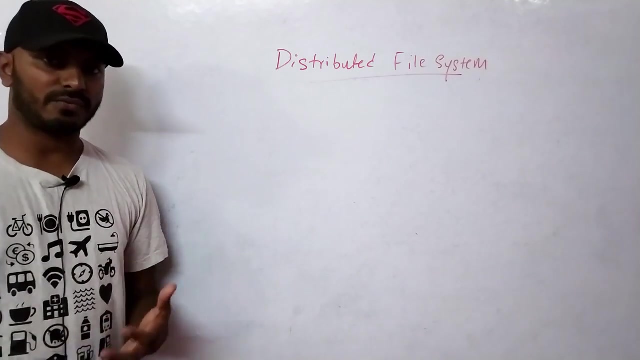 sector where that file is present from the storage and it basically retrieves or writes there at any time when you write and read, and also a lot of file system does use a lot of compression techniques to save these files into the disk, to save a lot of, you know, memory and all of that stuff happens and it 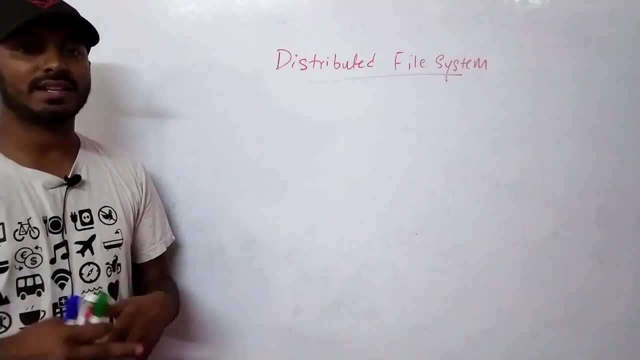 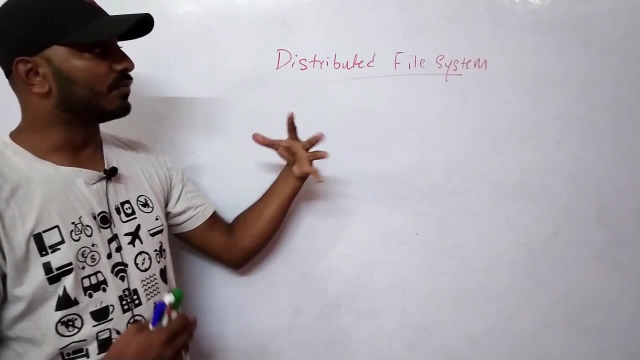 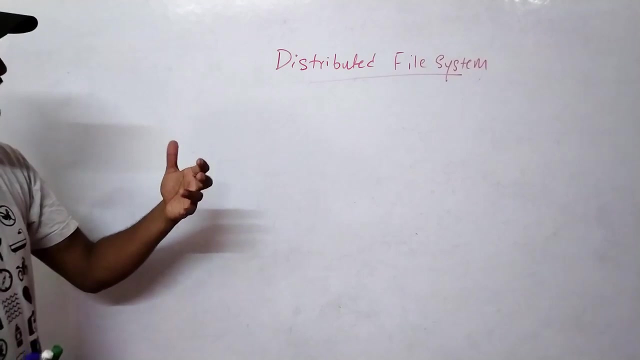 also handles the- you know- directory structures and the naming conventions and everything you don't need to really understand about the internal working of the file system. but we need to understand a little bit, just just for the sake of it. so let's jump in why we need a distributed file system. 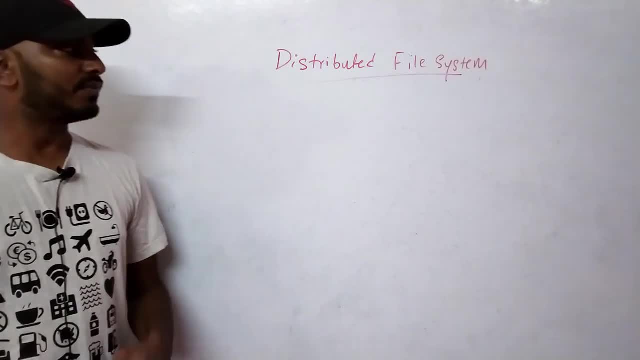 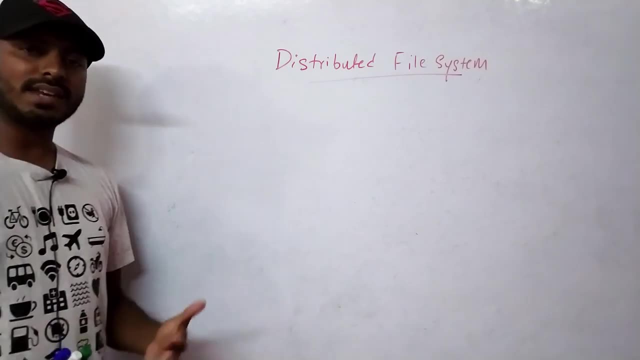 and how basically distributed file system works. there are a lot of distributed file system and I'm going to take one example and explain how that works. let's understand why we need it first. okay, so now let's take an example to understand why we need distributed file. 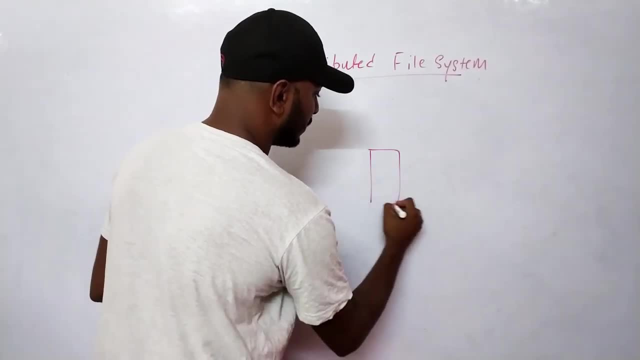 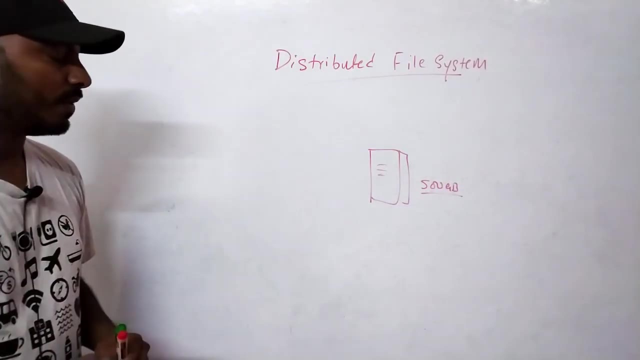 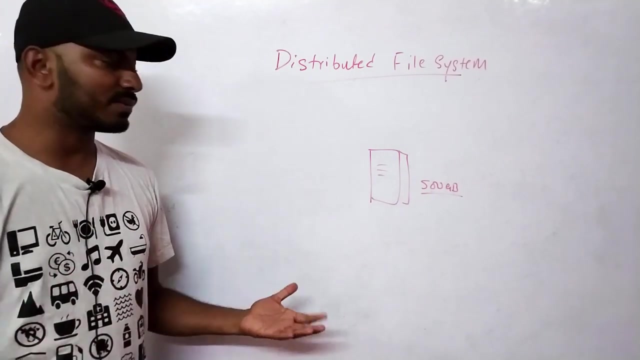 system. say suppose I have a CPU with about 500 GB in it. how did you be hard-disk in it, so I can only save files up to 500 GP? but think about it: we might have files more than 500 GB, right? what if I have files? 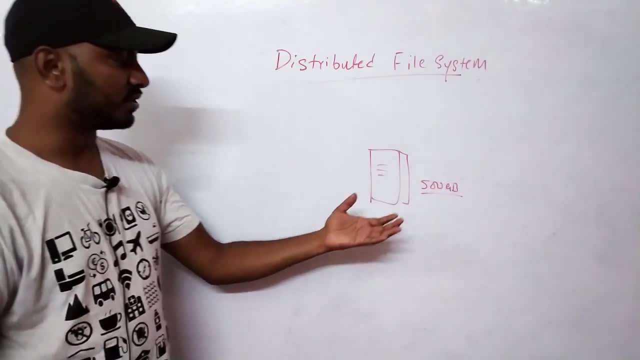 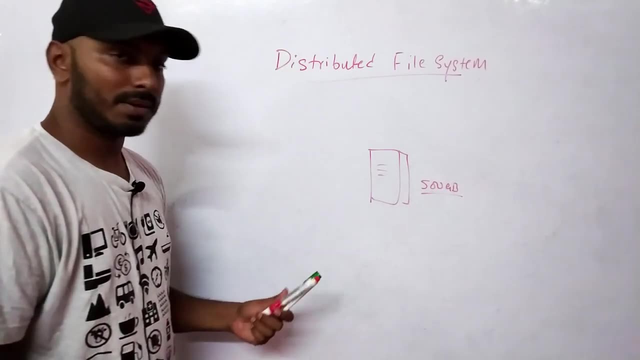 of about 700 GB. and then how do I save it to this server? it's not possible because I only have 500 GB. all I have to do is either upgrade 500 GB to maybe 1 TB, maybe buy a new hard disk of another 500 GB, or replace the old 500 GB and get. 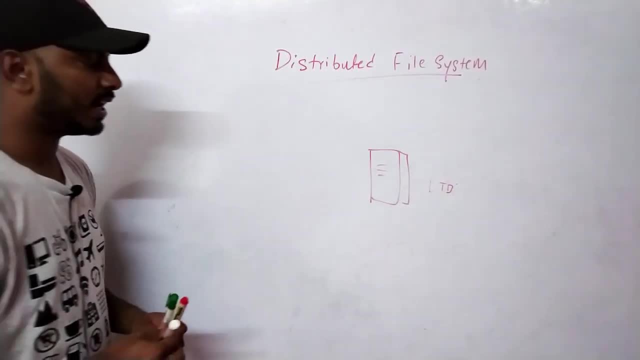 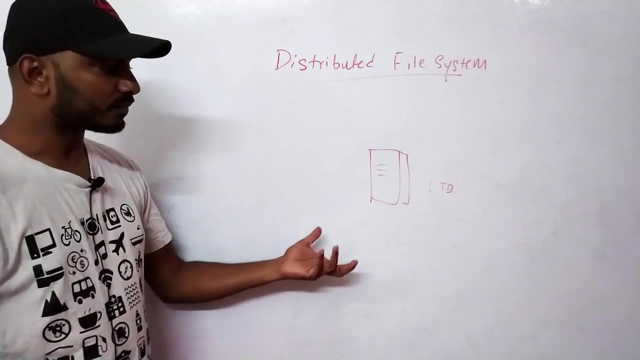 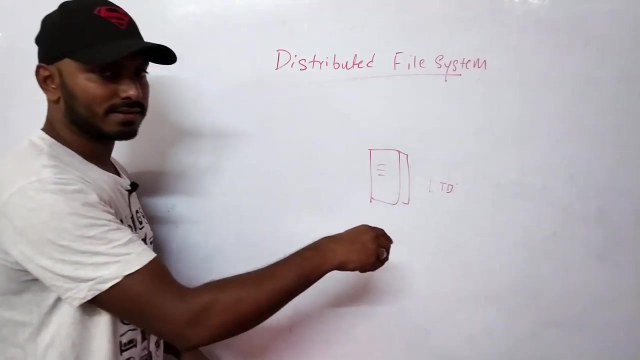 1 TB hard disk and have that available in the server and I can now save up to 1 TB of files. what if I have, okay, 10 terabyte of file? what do I do? so I have to. I will have to buy 10: 1 TB hard disk and attach it to this machine. but this 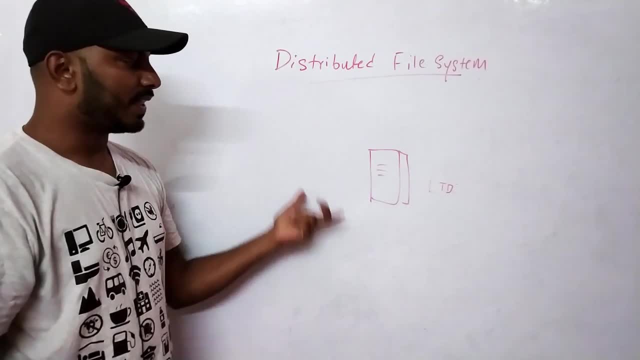 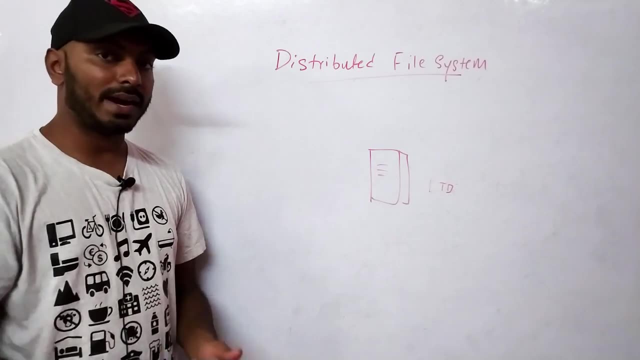 machine may not be able to support, then I need to buy a even powerful machine to support. you know, 10, 1 TB hard disk. or I will have to buy 10 TB 1 hard disk and that will be much more costlier than buying you know. 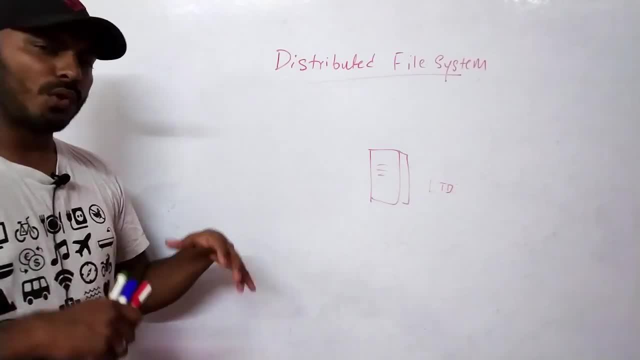 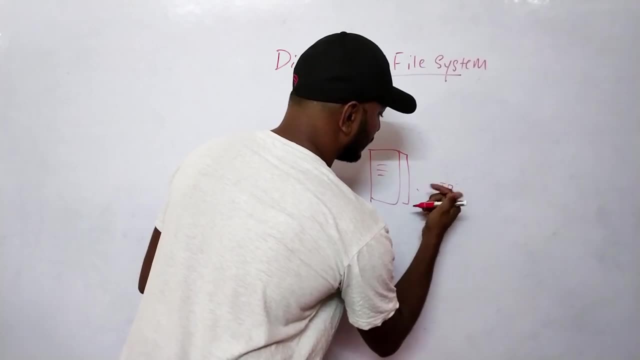 10, 1 TB hard disk and that will be much more costlier than buying, you know, 10, 1 TB hard disk. so it's all not feasible. so think: okay, I somehow upgraded the machine and I was able to upgrade this to 10 TB. okay, and then I'm saving all of. 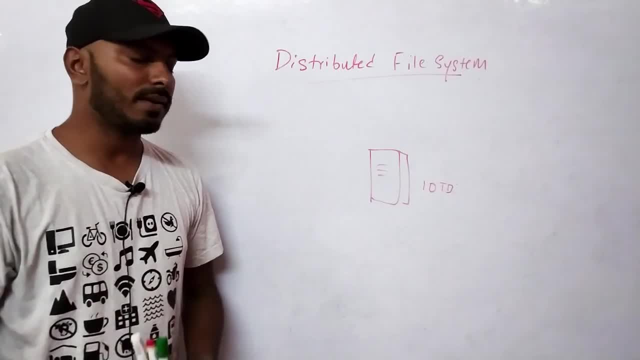 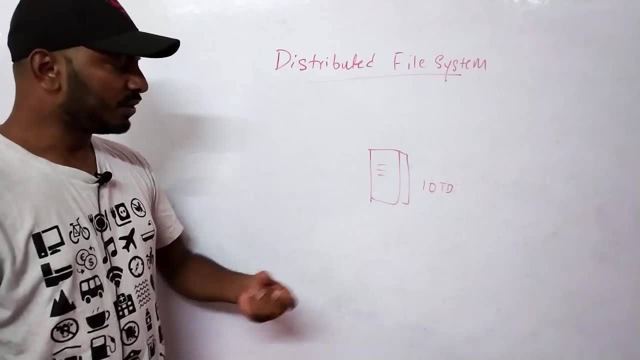 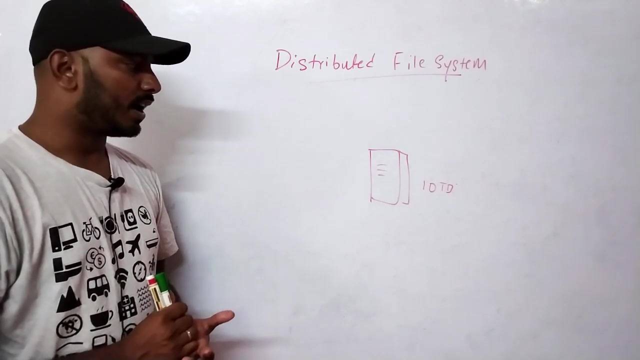 that data or files in this machine. okay, now all good, so happy scenario works. what if, for some reason, those files are very critical or very, you know, high, of high importance, and I don't, I'm not supposed to lose those files now, if you see, this is like a single. 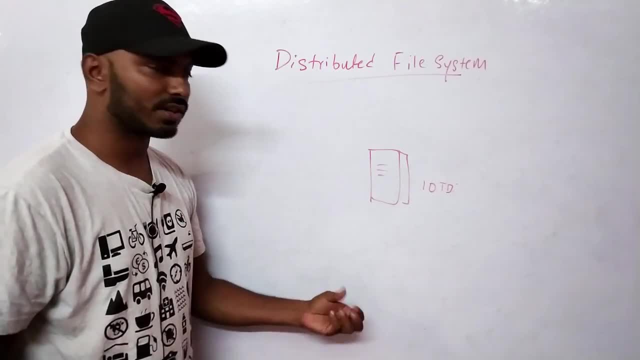 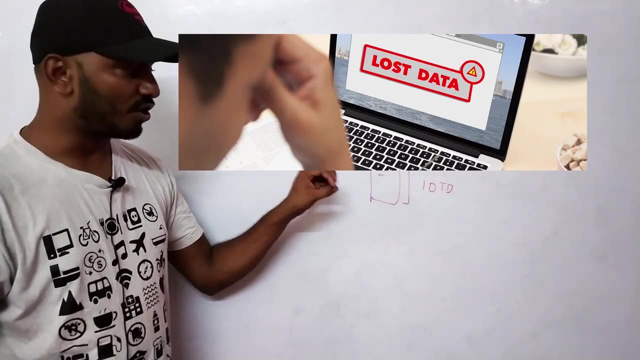 point of failure. what if this machine crashes or something, it caught fire or the hard disk failed? what happens to my data? all gone, right, all of my data is gone. now how do we make sure that we don't lose that data? so I'll have to buy. 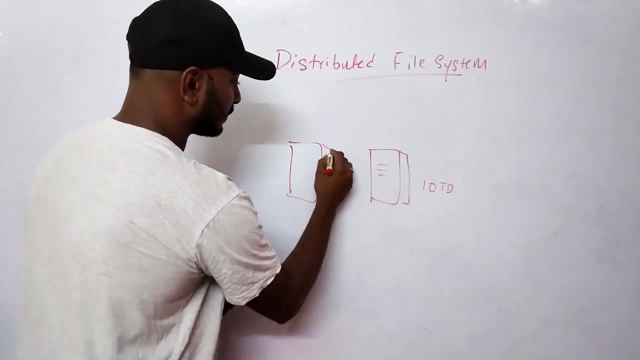 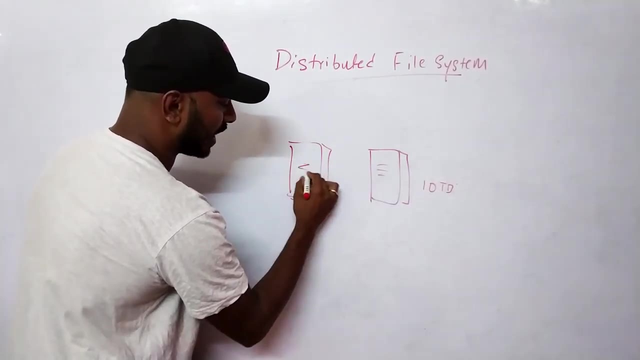 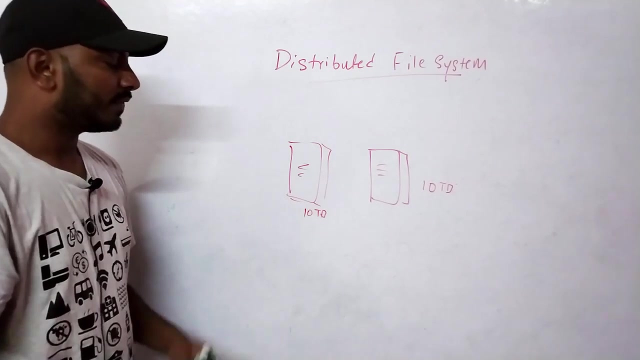 one more machine, or yeah? so transfer cop, keep a copy of all the you know data which I had in the server to another 10 TB of files. you know, another 10 TB of hard disk. that way we are safe now, even though if I lose one machine, 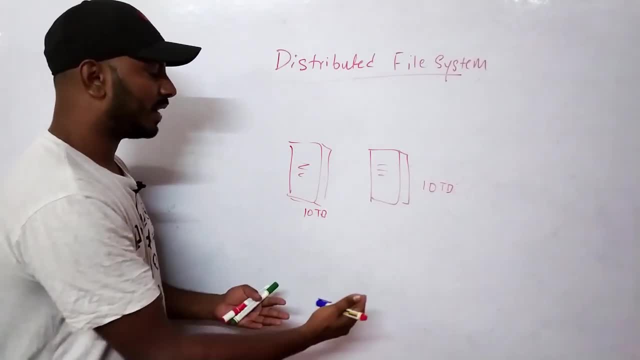 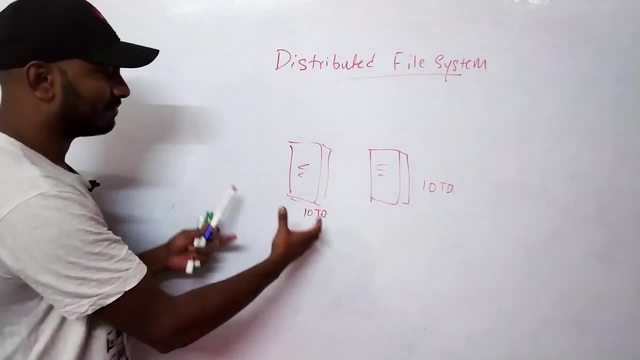 I have all of the files, so I have all of that files saved in another machine. so I'm safe now. but I can't always keep on buying machines like: okay, tomorrow if I need another 10 TB, I'll have to either upgrade this, then I need to upgrade this, and then I need to upgrade. 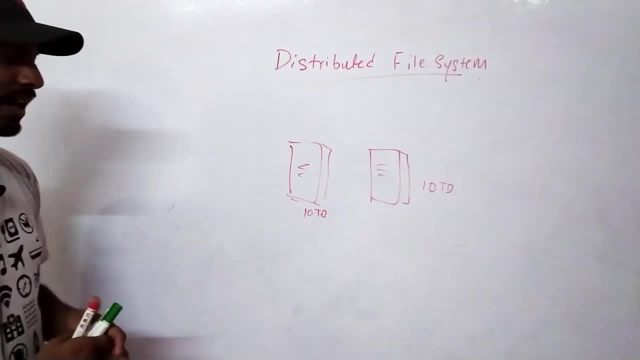 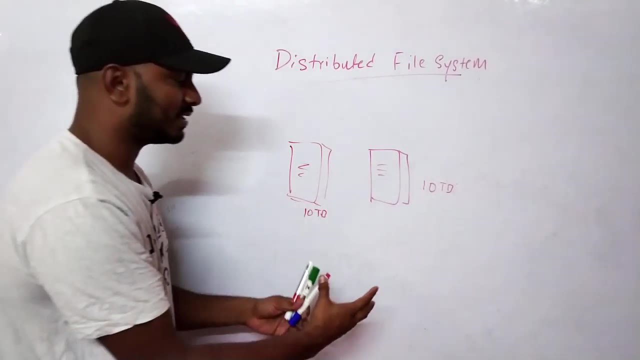 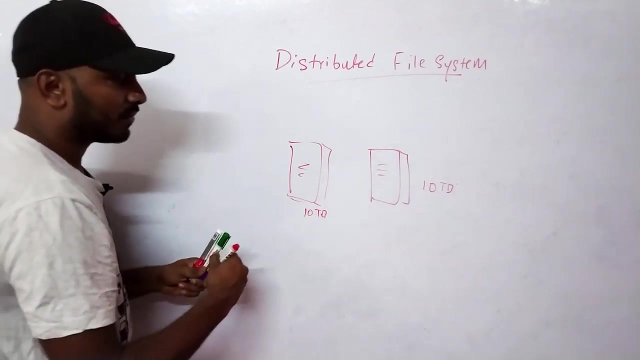 this as well, or buy one more machine. it is like getting out of hand and it is like a totally unorganized way of doing it. what if I had very small files of just one KB? and then I'll put millions of files like: how do I transfer it here? what if I upgraded this? 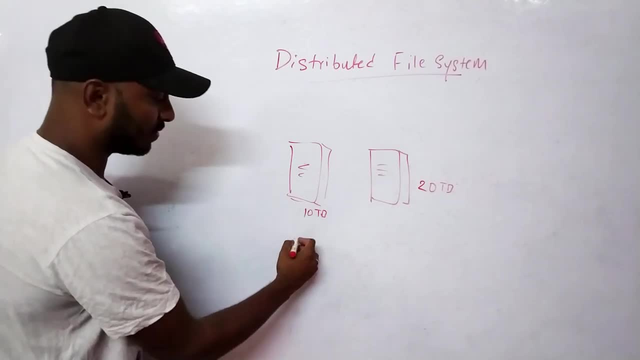 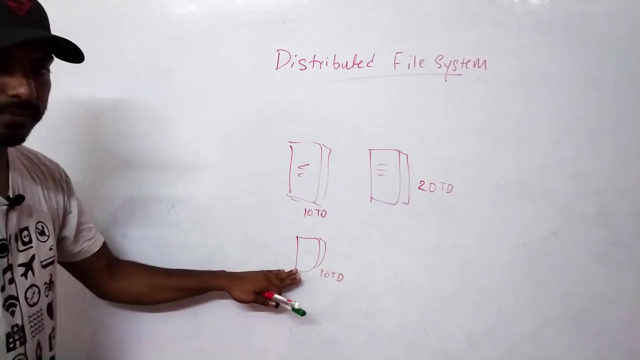 to 20 TB and I need to either upgrade this also or I need to buy one more machine with another 10 TB and then copy here, copy half here and copy half here, and so this is totally unorganized, because when I want to search that file, how do I know? 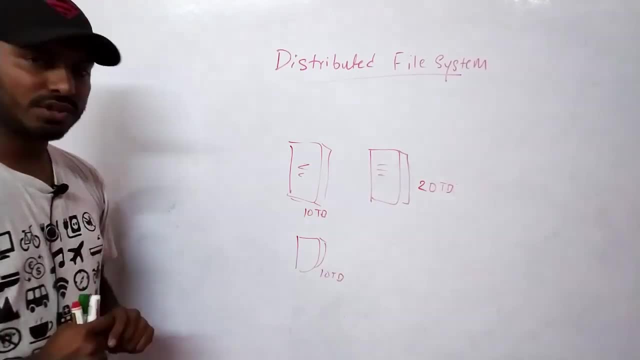 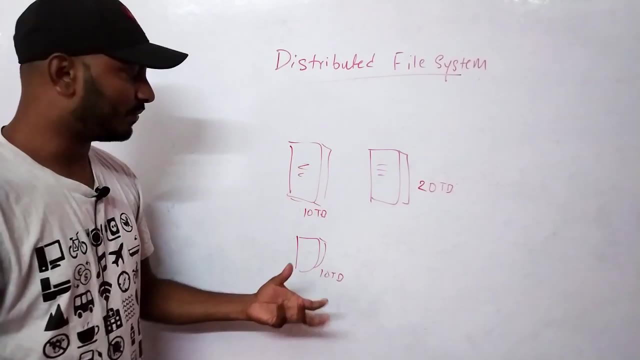 where those files are. maybe this got crashed now. I know that for sure some. you know files are backed up in this machine and this machine, but I don't know really where that file is here and where that file is. where there are two machines. maybe if I had more machine I 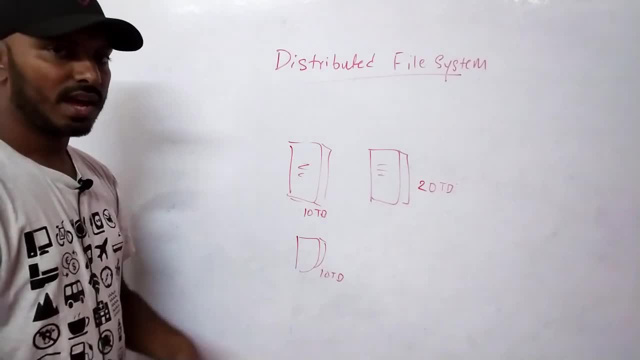 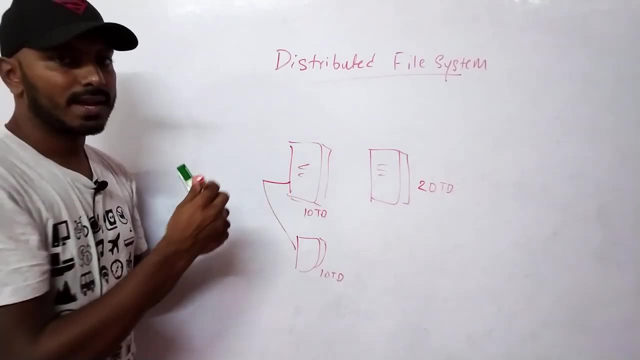 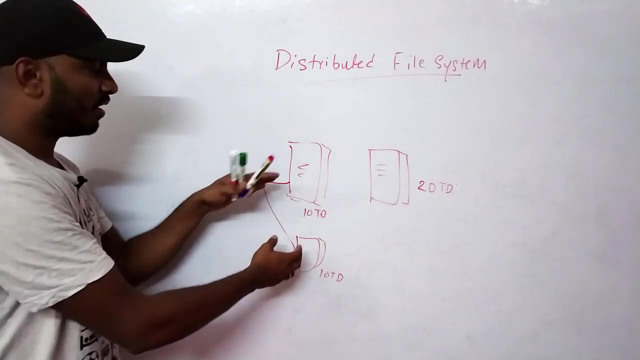 don't. it's very hard to find those machines. otherwise I will have to connect all of this machine into one network and I can access from one place. But that is also difficult because I need to keep on logging into these machines, or you know all of these like a network file, old way of doing it. right, that's that, doesn't. 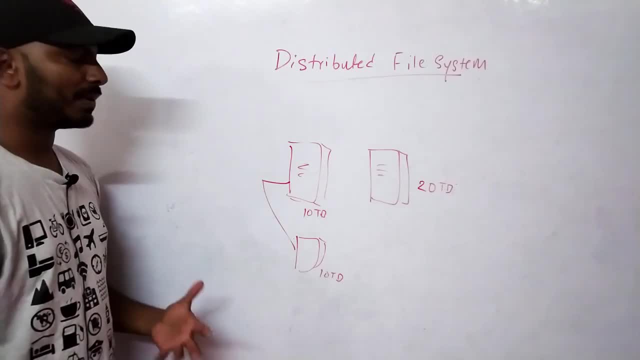 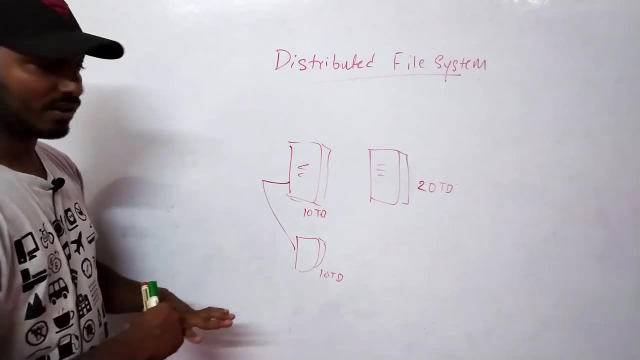 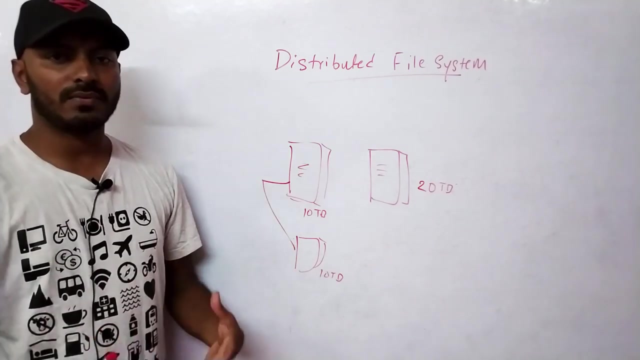 look good, but definitely when we are in the big data era where we have, you know, petabytes of data. in that case, doing this way is is not a really good idea. so that's the reason why we need distributed file system, Because the conventional file system which we had, like NTFS or exFAT or FAT, were basically 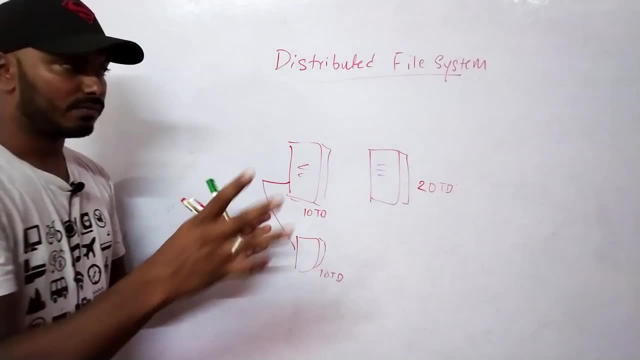 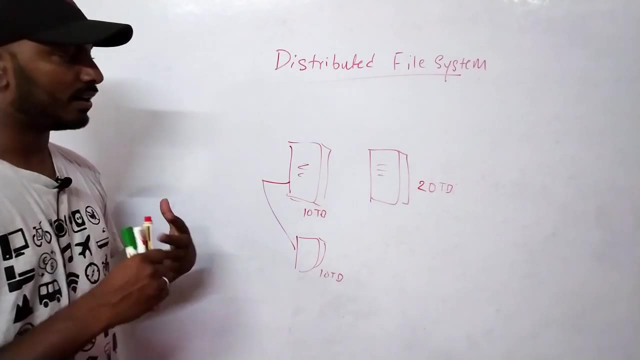 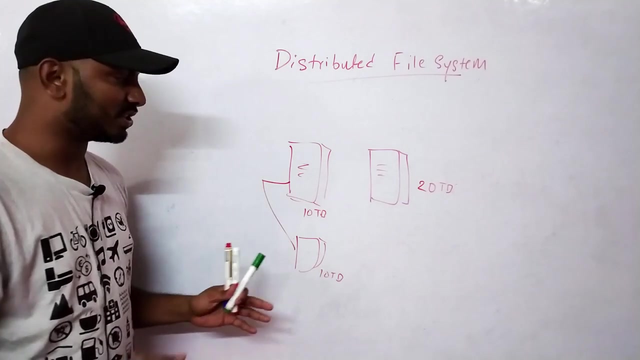 designed to handle only one machines. you know data storage needs, but not across the machines. So distributed file systems are, you know, brand new. you know file systems where they are kind of designed to handle across the machines, not just. they just don't worry about one machine. 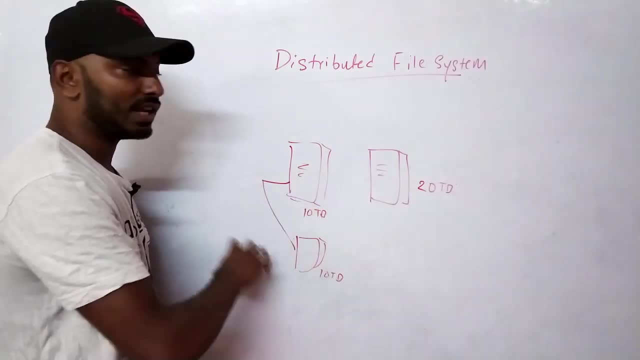 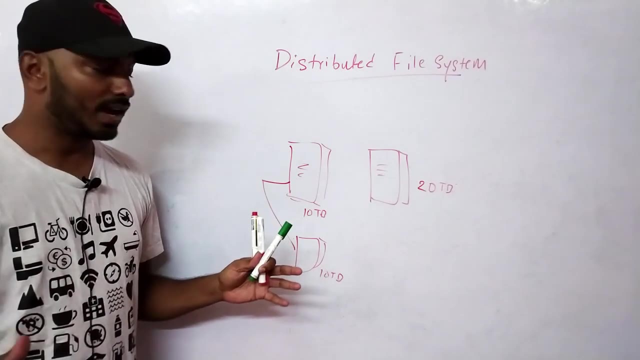 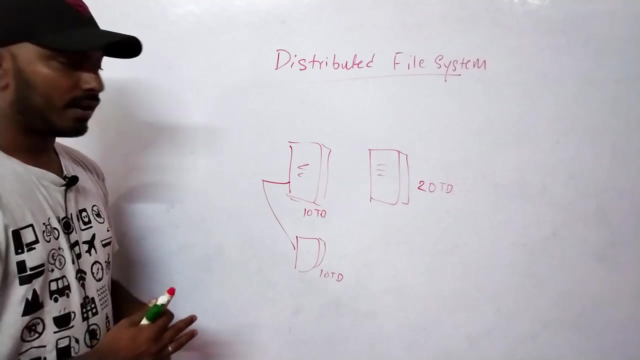 they basically understands all of the storage Availability in all of the machines in the cluster to, you know, form of one big hard disk so that we can seamlessly upload a file and then we don't need to really worry about where that file is. Just to give an example how that works, let's take in a cluster. consider we have three. you 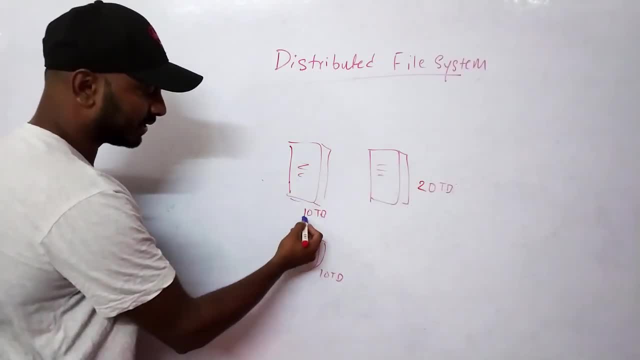 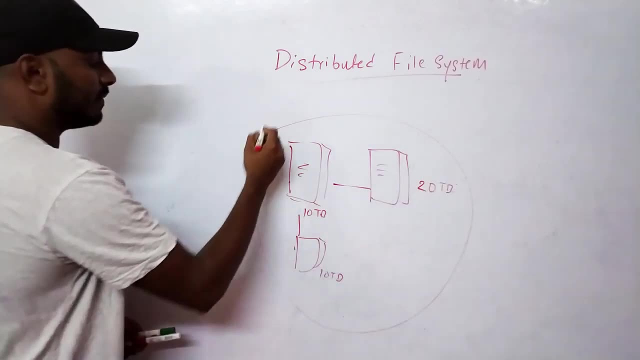 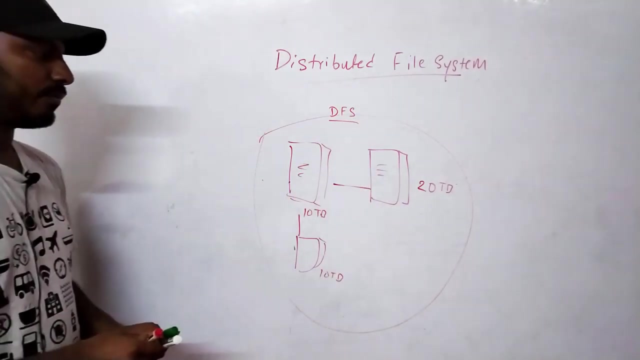 know machines, yeah, so same thing: 10 TB, 10 TB, 20 TB, and all of them are kind of like interconnected. And now let's see, let's say that this itself is a distributed file system. Now, if I have a file of about you know, 35 TB, how do I store it? 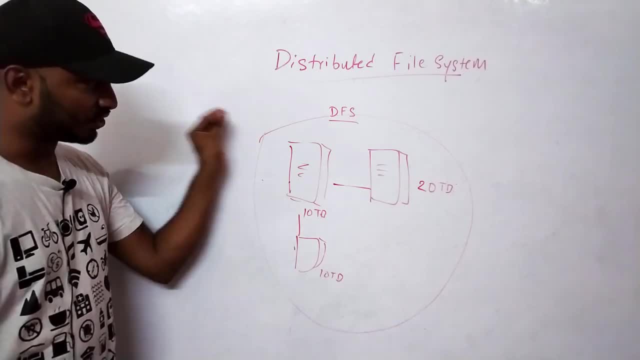 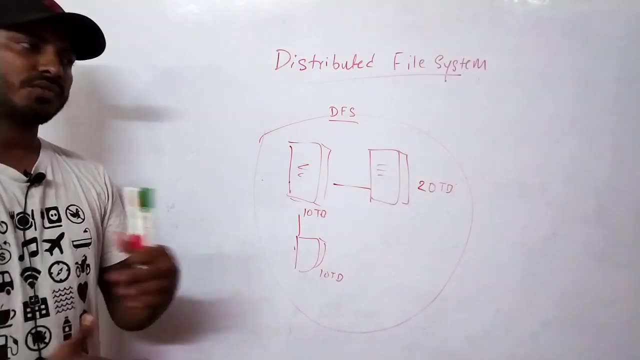 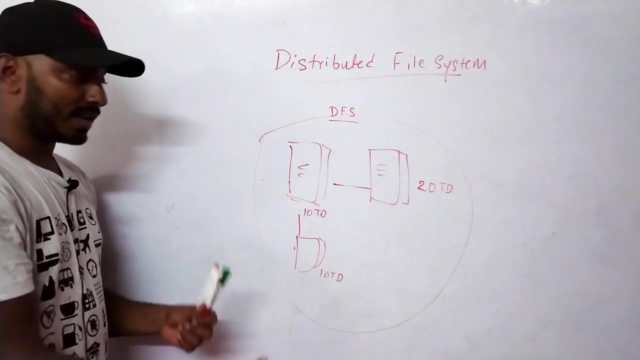 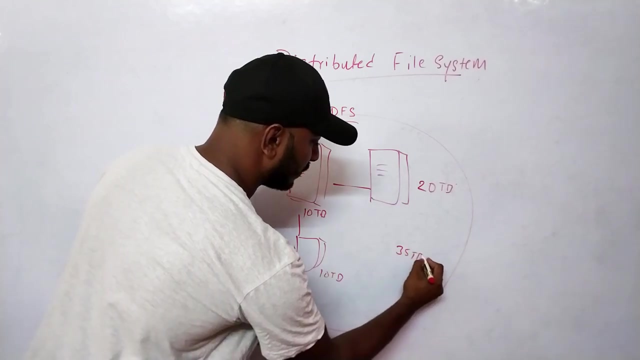 So when I, you know, copy that file into distributed file system, what happens is distributed file system automatically breaks them into chunks, like about 64 MB blocks, and then it automatically keeps on filling wherever it is possible, wherever there is space available. even some files were already here. so, as I said, I think I said 35 TB, right. 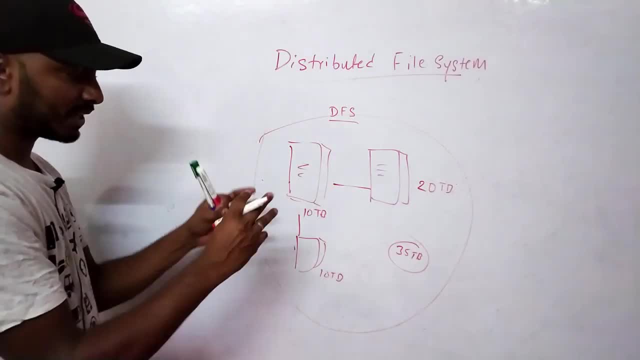 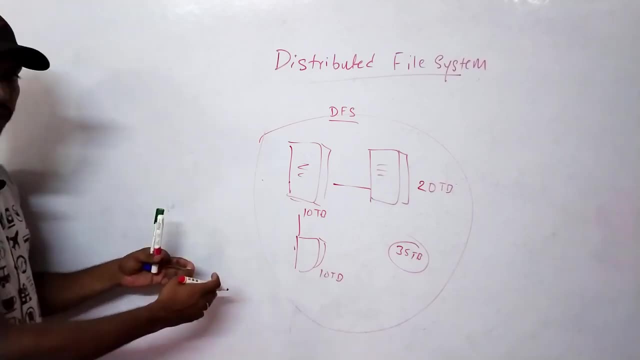 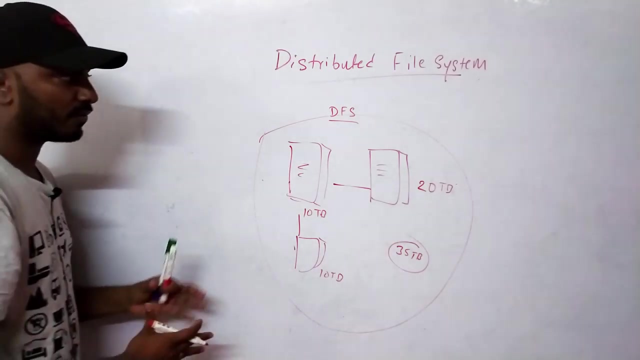 One file- think it 35 TB of one file. it breaks into small, small chunks and then it stores wherever it is possible. But when I query for that file, it automatically knows where are those chunks placed in all of this machine and it retrieves and gives me as one file. that's the beauty of distributed. 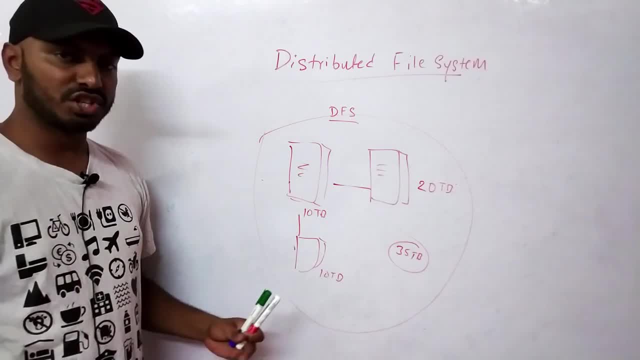 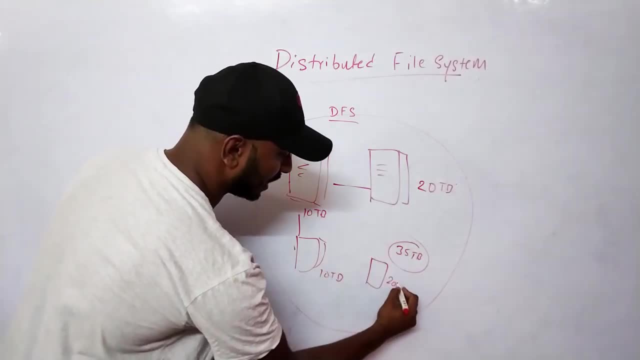 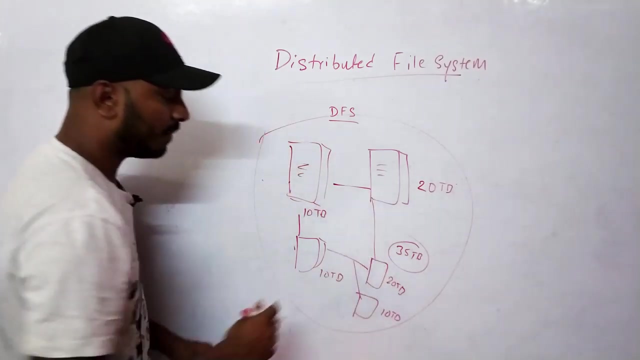 file system And also I can specify the replication factor. that means that, provided that there is enough space here, maybe I had one more machine of about 20 TB and one more machine of 10 TB. so now I have so much of storage available in my network. 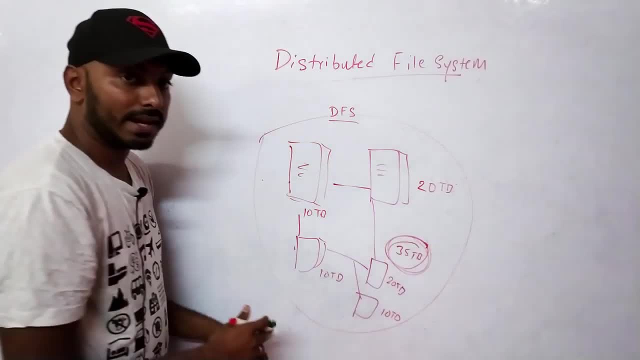 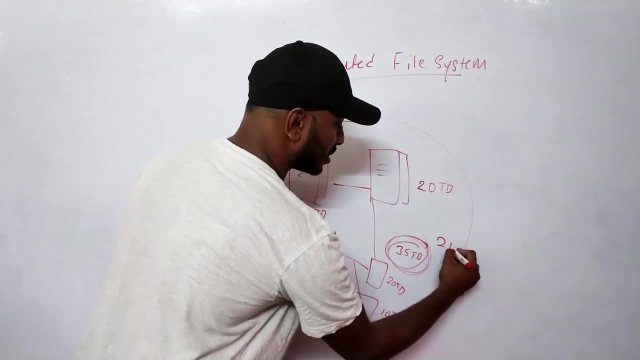 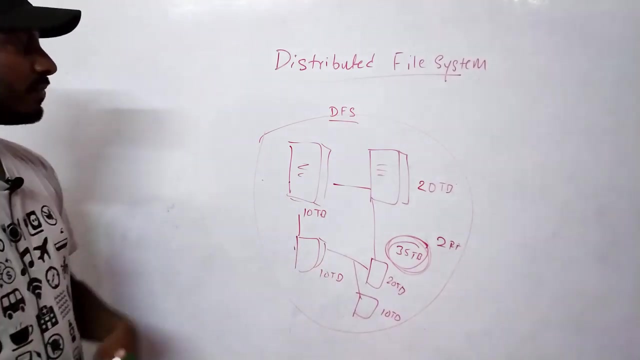 Now if I copy one file of 35 TB and I say please replicate into two copies, maybe set it to two in a replication factor, That means that there are two copies of the files in these machines. So distributed file system is so clever that it automatically arranges in a way that even 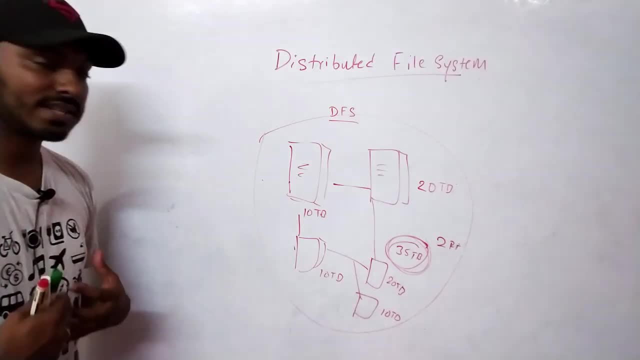 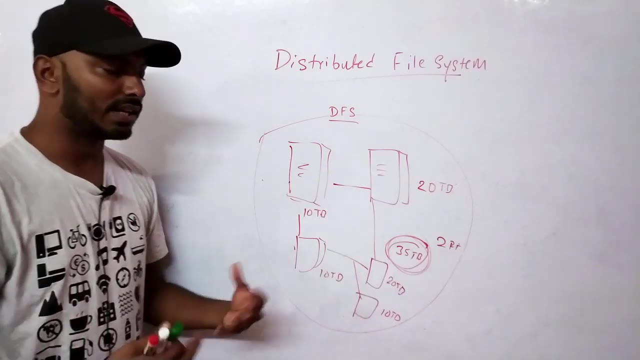 if we lose couple of machines in these clusters, we still get that file, all of the pieces of the file, intact, so that I can still recover that 35 TB file as a whole. That's the beauty of distributed file system, And in these days. 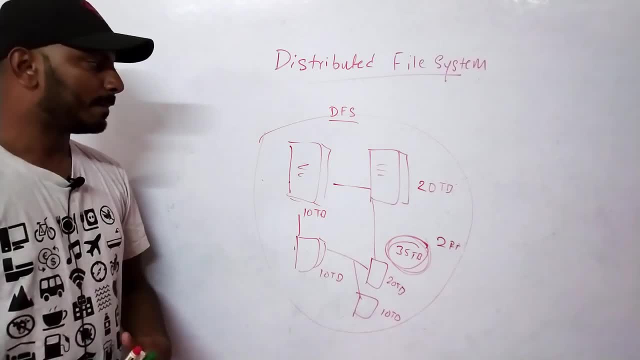 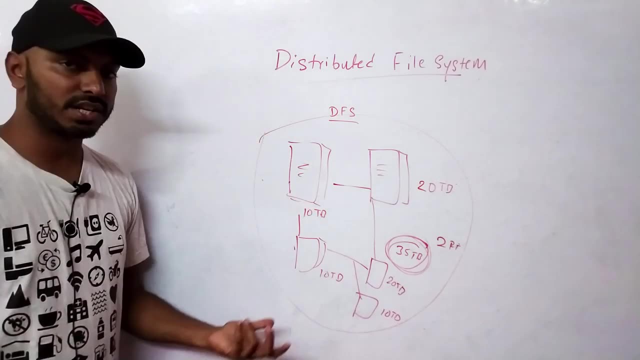 We really need this distributed file systems because of big data. we have so much of data and we know that we are using commodity hardware. they are not like super computers, they are just a commodity computers which we all have at our home, so they might fail at any time. 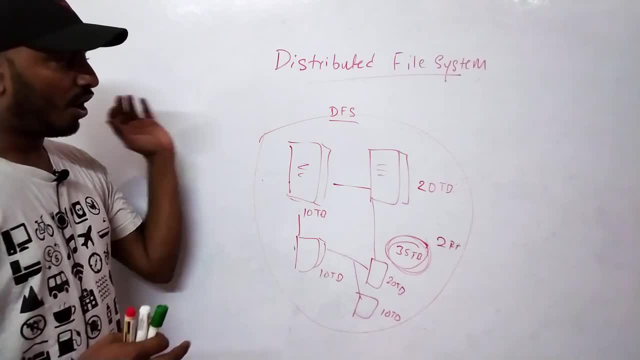 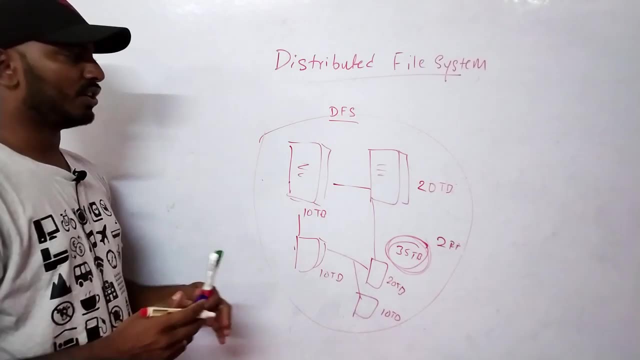 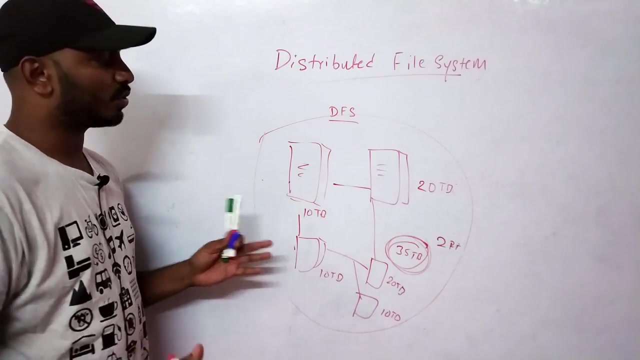 so we are not afford to lose that data. so all that logic is embedded to distributed file system. So namely, some of the distributed file systems are: you know, HDFS, that is, Hadoop distributed file system, or I think even Gluster file system also works something similar. I'm going 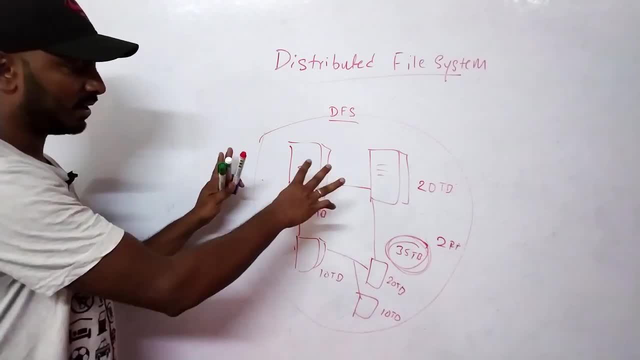 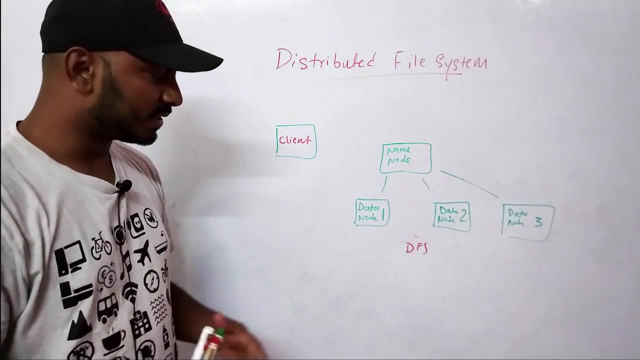 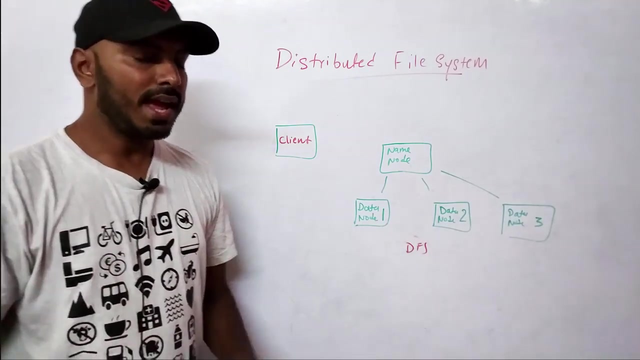 to explain, like how basically the distributed file systems handles when we write and read. okay, so this is how the distributed file system look. distributed file system, like basically HDFS, has two main components to it. one is name node and one is data node. name node, as the name itself indicates, doesn't actually store the data of the actual files which we 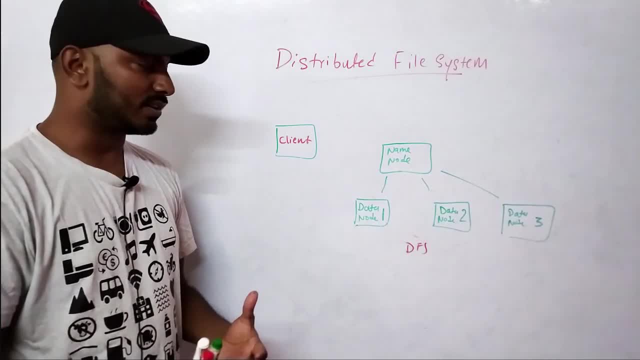 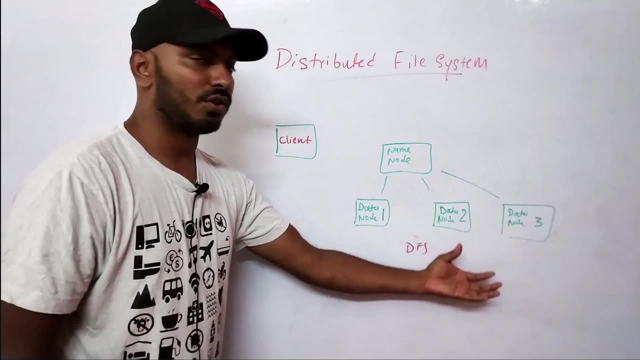 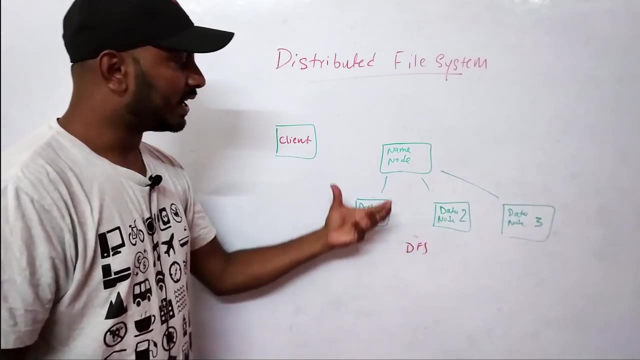 want to stay, But instead it is the one it acts like a master. basically it kind of knows the information about where the file is in the data nodes. basically it is the one which actually checks the health, health check of all of the data nodes and it also has the information of what 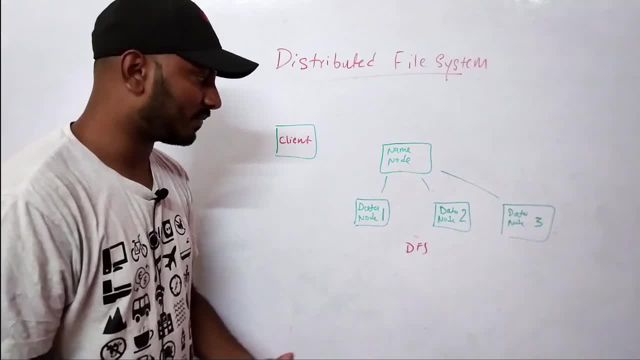 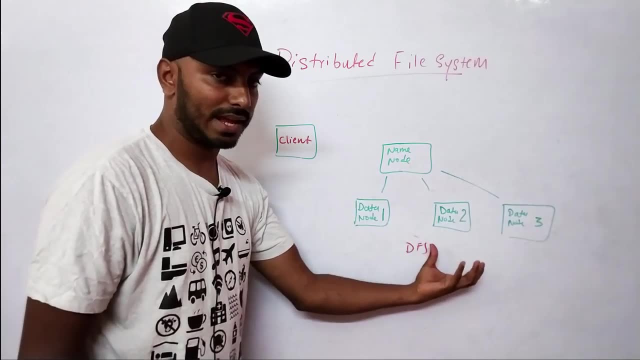 is the size of you know data node and how much it is filled and how much it is empty, and all of that. and it also takes care when machine fails And how to move the data in between other servers so that we still have a copies of. 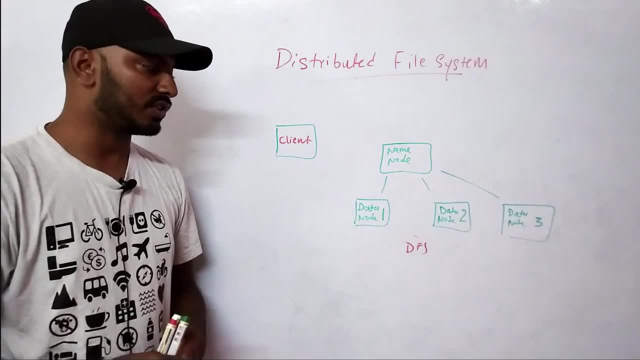 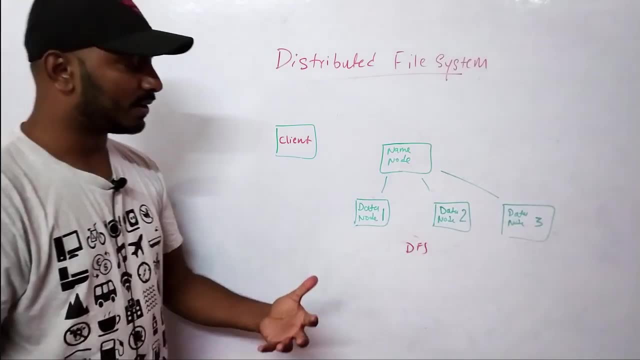 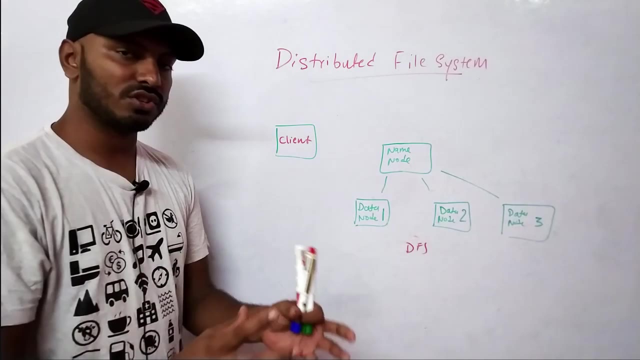 the files according to the replication factor which we have set. and there is one more thing called, as you know, blocks size, which we can configure. Let's say, it is configured for 64 MB block. That means that, as I mentioned, any file which we tried to upload, it will be broken down. 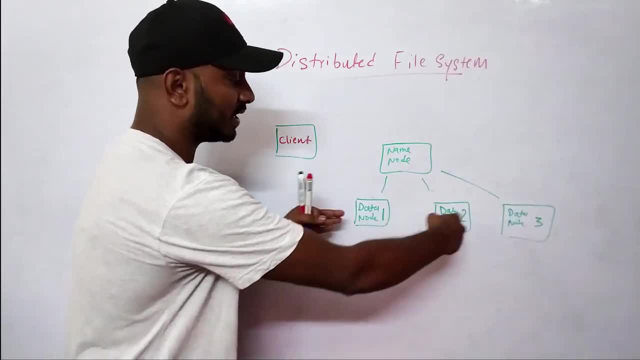 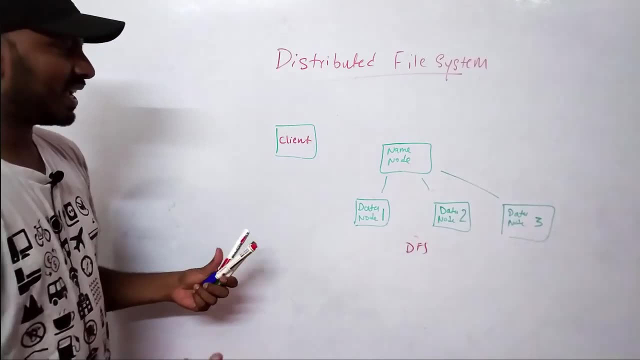 into 64 MB and then they will be distributed across the different data nodes so that we have the redundant copies properly. So there you go Now. I hope you guys have enjoyed this video. I'll see you next time. Bye, bye. stored in the available space. so let's see how basically the process of saving. 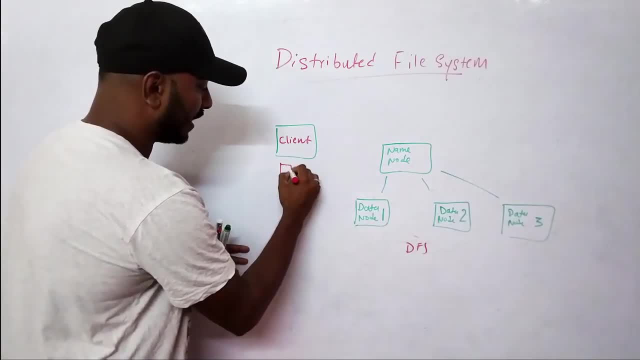 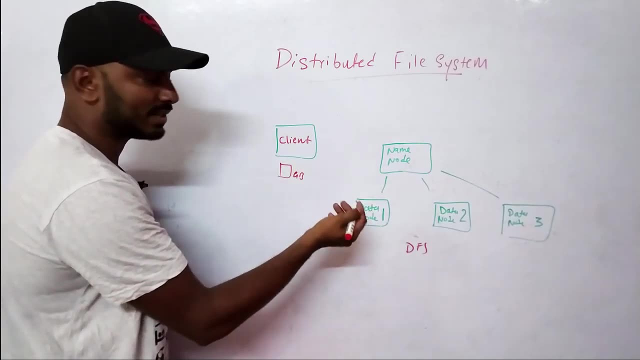 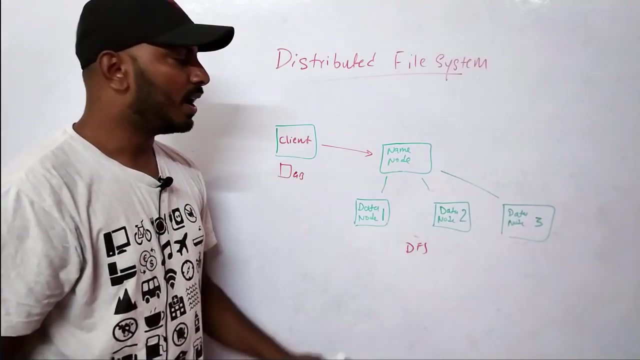 the file works. now I have a client and I have a file which I want to save. maybe this has about, like couple of you know, GBs in size. it basically talks to the you know distributed file system first. it has to talk to name node. basically we. 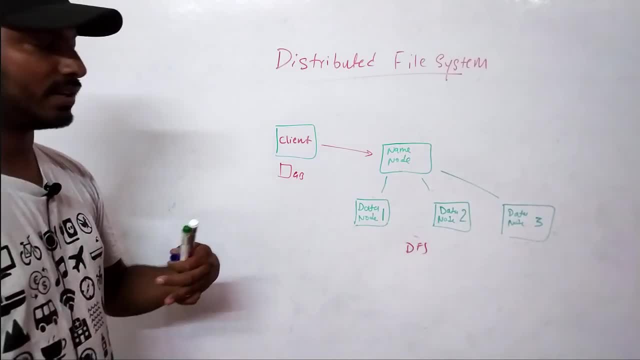 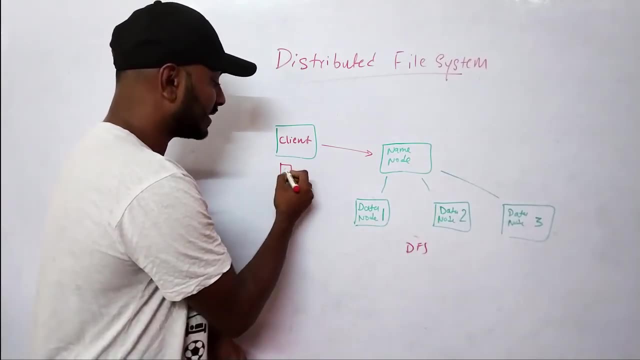 have a client library which is used to access the data and write and read. it talks to name node and say, okay, I have a file to write, it is of the size about 5 GB and where do I need to write? so the name node exactly knows the information. 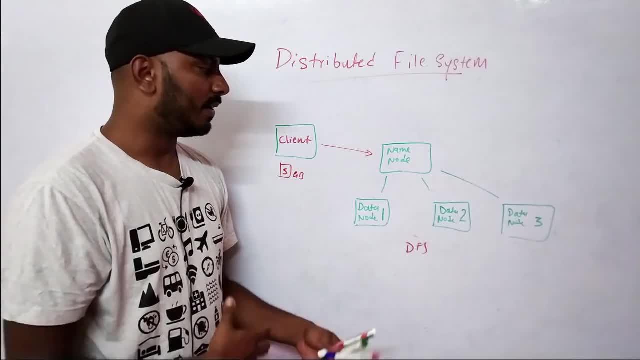 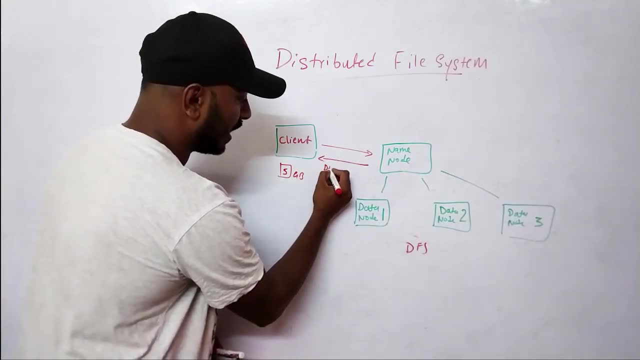 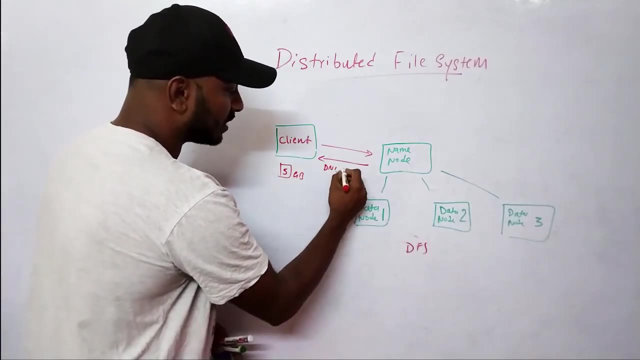 of about which node is free and everything. so it basically replies back to the client. okay, please go ahead and write it to data node 1 and tell the data node also to replicate it to data node 3. so that's the information it basically gives it to the 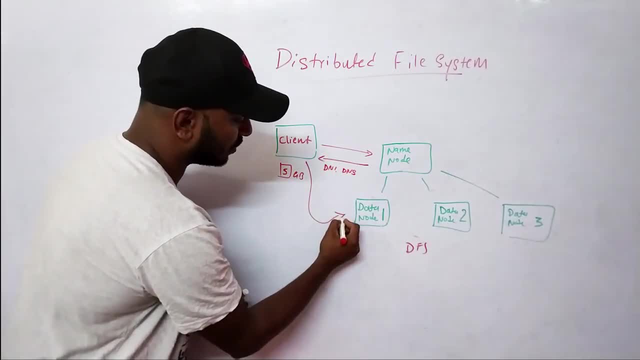 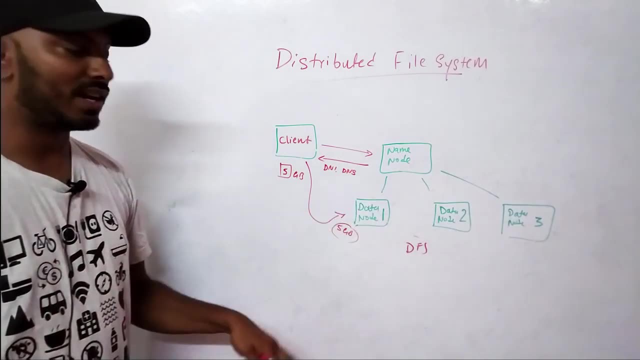 client and then the client go ahead and write to data node 1 of all the 5 GB here and then it also tells: okay, the name node has told: please write it to data node 3 and the data node 1 will take that responsibility of replicating. 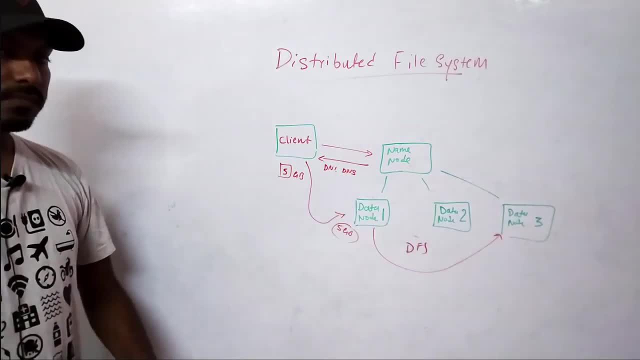 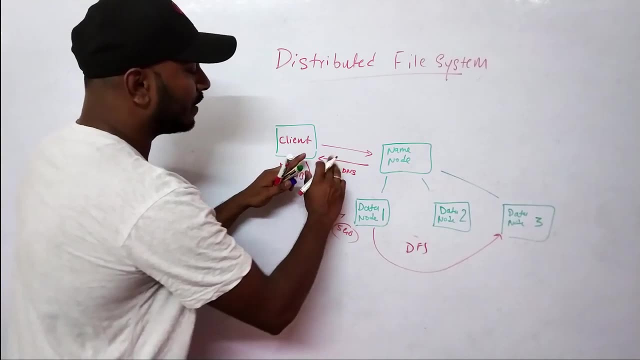 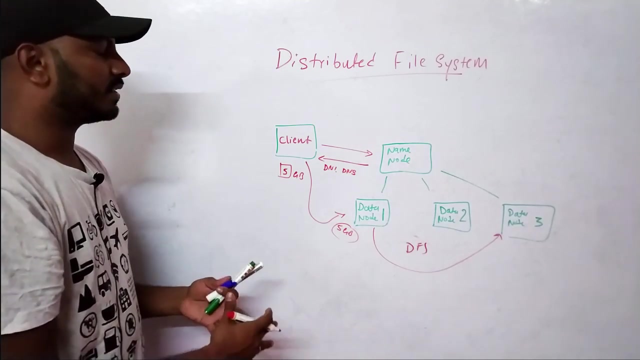 all of that information to data node 3 automatically. there could be some other you know distributed file system where this whole interaction will be taken care by the node itself, but this is the. this is how the generic data distributed file systems works, where the name node has all of the meta. 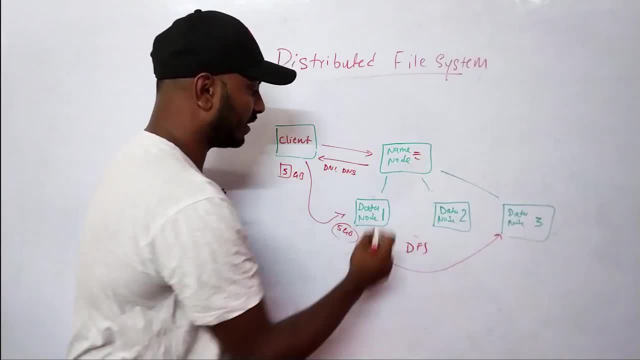 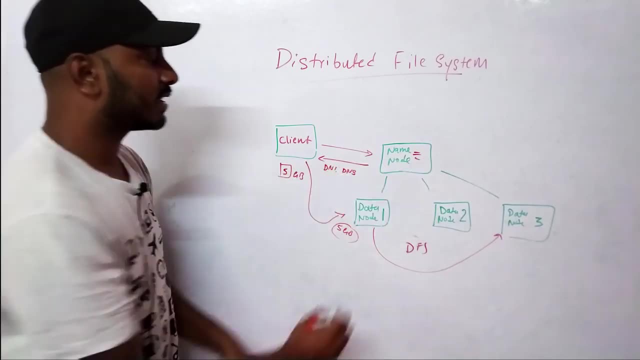 data information of where the file is and also it is going to record that. okay, this file will be presented in data node one and the copy is presented in three. so that's that. name keeping job will be taken care by name node. so now we have the 5 GB. 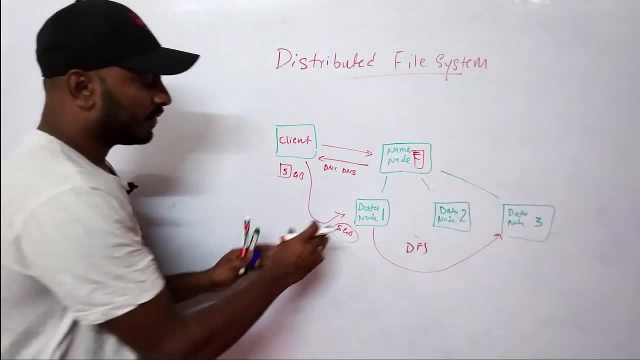 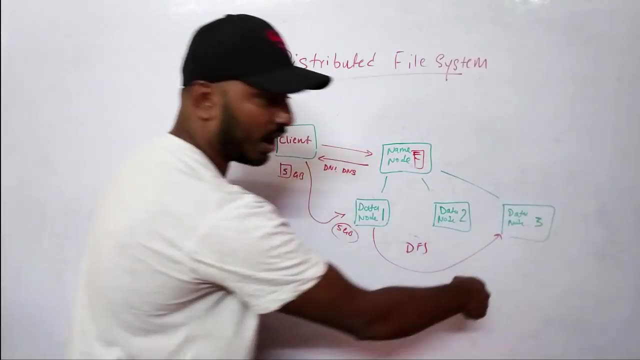 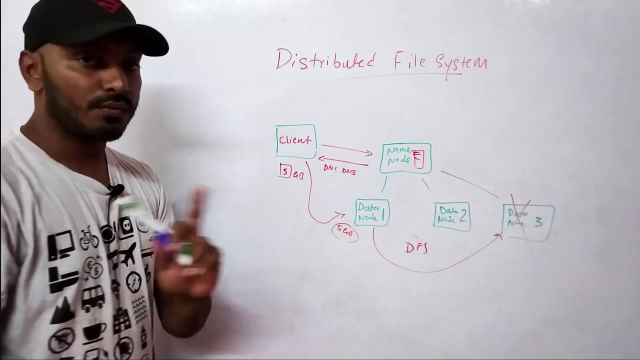 thanks for your continuous support. you know file saved in data node 1 and 3. for some reason, if this machine goes down, then we know that the copy of 5gb which we just wrote is not available in the system. we just have one copy and we're not supposed to just keep one copy because if this machine goes down we don't have 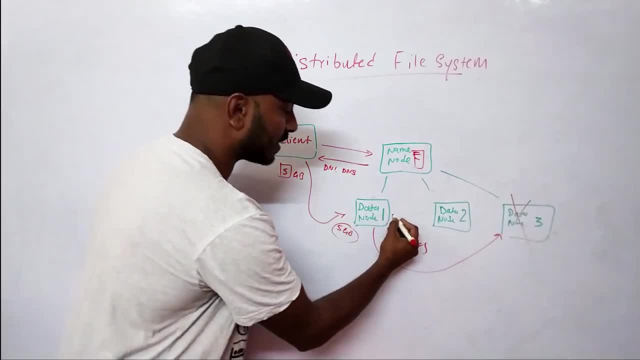 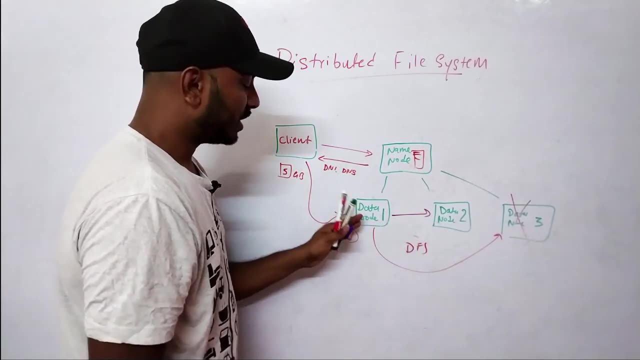 the file at all. so the name node automatically tells the data node: please replicate to the available data node if the space is available. so now the data node will know that. okay, i need to replicate it to data node 2. so it basically copies all of the 5gb file here in the data. 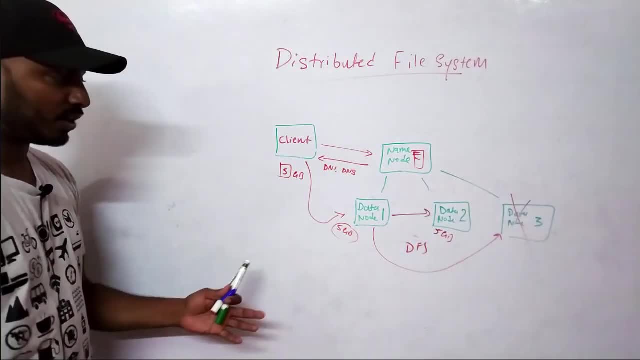 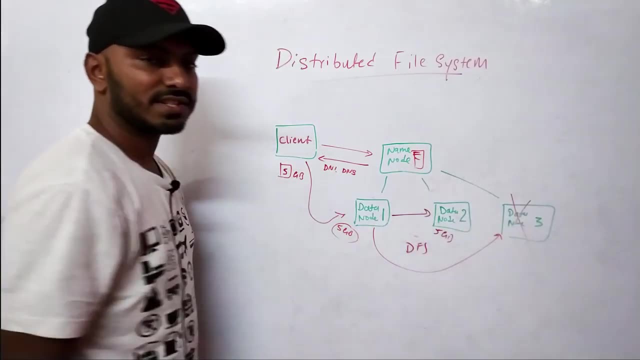 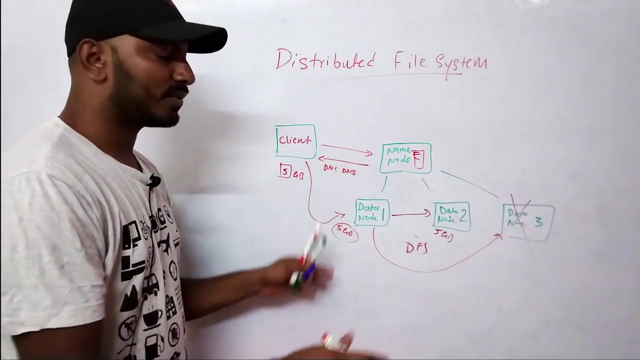 node. so we still have two copies in the system, no matter what. even if one machine goes down, we still have that file gb somewhere here. but on a worst case, if all machines goes down, i mean obviously we will not have have the data, but most likely we won't have that kind of problem. 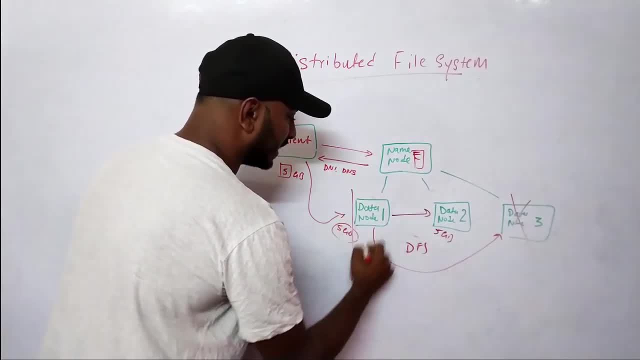 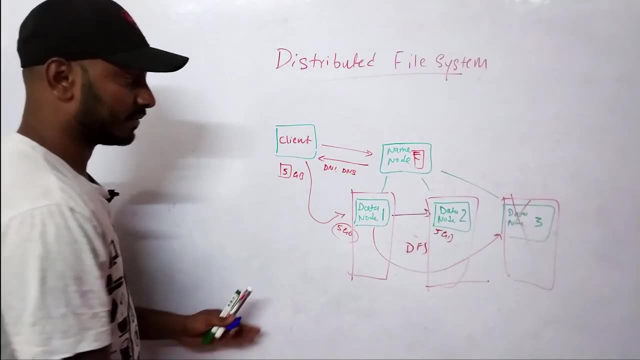 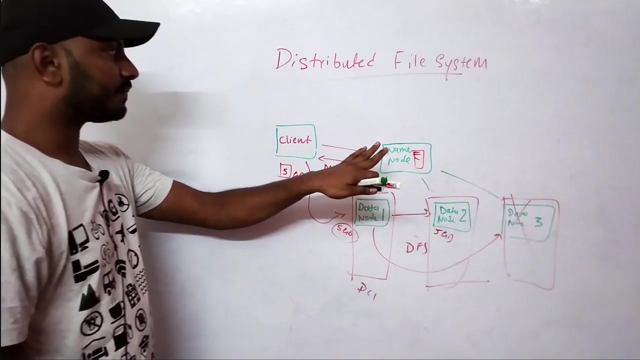 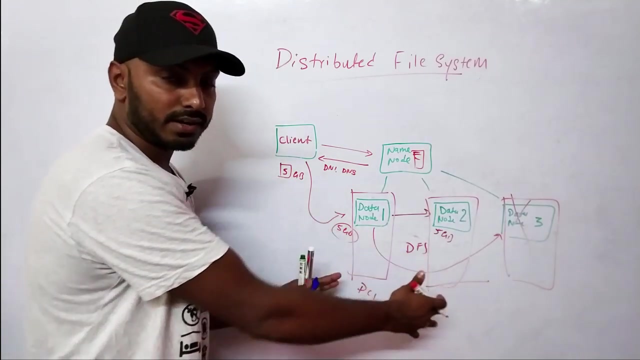 because so most likely we'll be having these data nodes in different rack and also we'll be having in different data centers itself. maybe this itself is in data center, one which is in some location, this in some other location. so this distributed file system also understand the- you know data center aware and rack aware, so they know that the replication 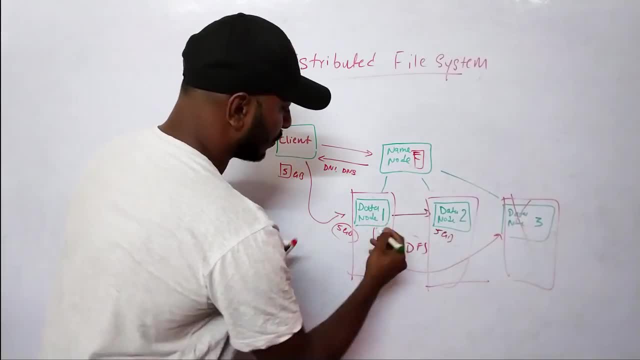 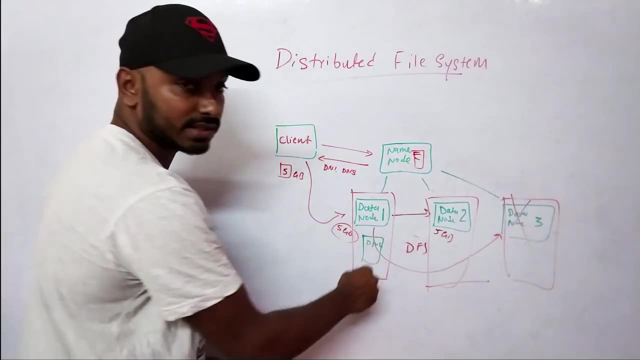 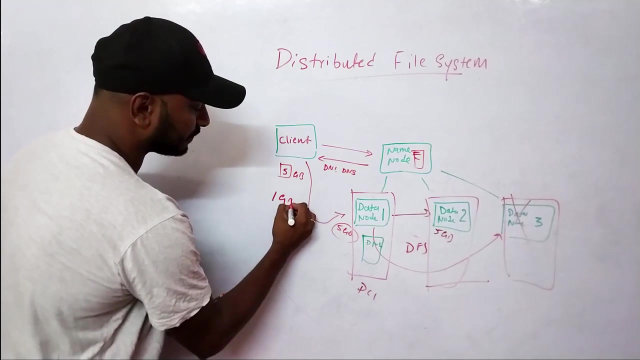 shouldn't happen. in the same rack. maybe there could be one more node called as data node four. it it most likely avoids not to replicate here itself, because if this say, suppose this, i will write one more file here of one gb. so if the name node tells you to replicate it to one and four. 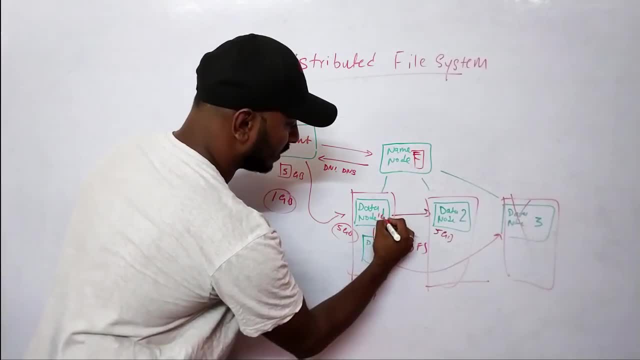 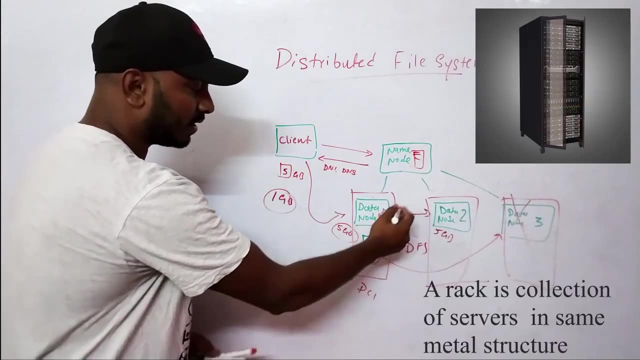 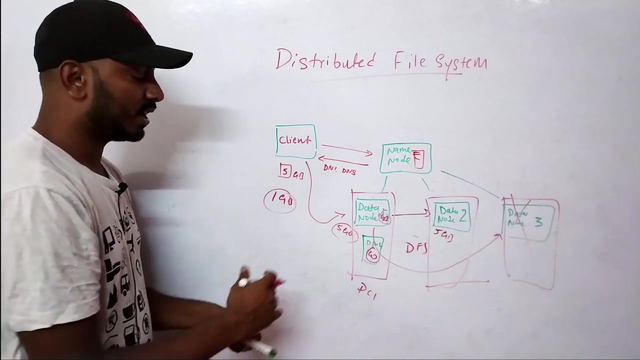 that's a bad strategy, because that one gb file is in here and also in here. okay, now what if this rack, which is in data center one, completely, you know, broken down or it caught fire? that means that both the backup and the actually copy both was destroyed in the same fire incident. so it's a bad strategy. so the distributed file. 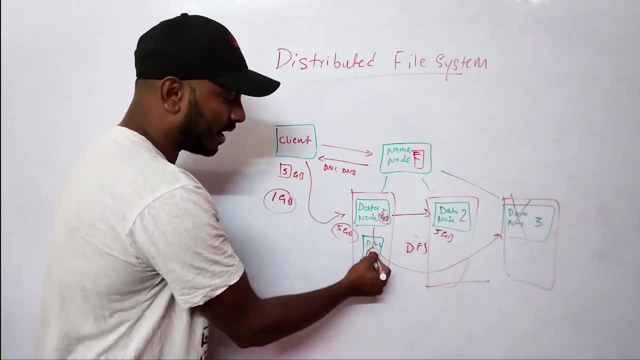 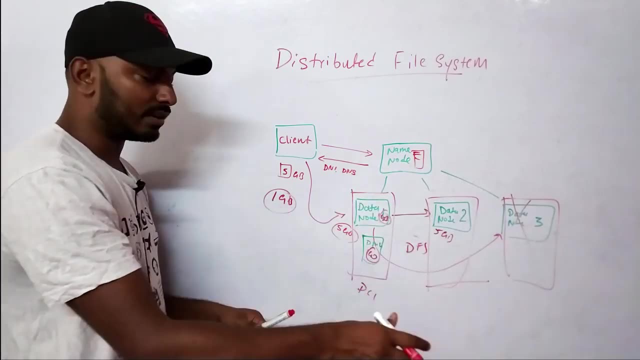 system also understand that i shouldn't be replicating in the same rack or same data center. it always tried to replicate into the cross data center and and then a different rack, so that way, even if one data center completely- you know- burned down, we still have the copies of the data in. 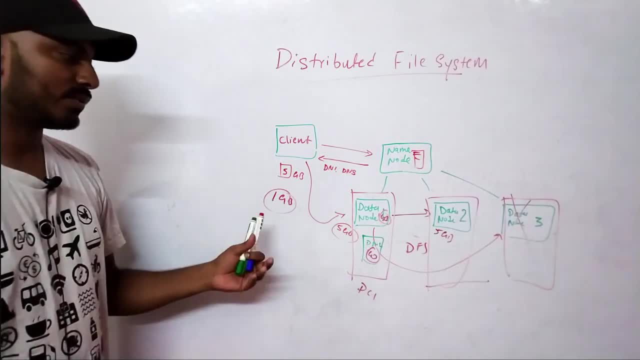 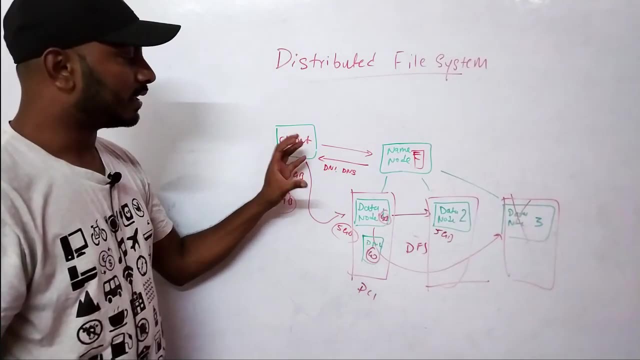 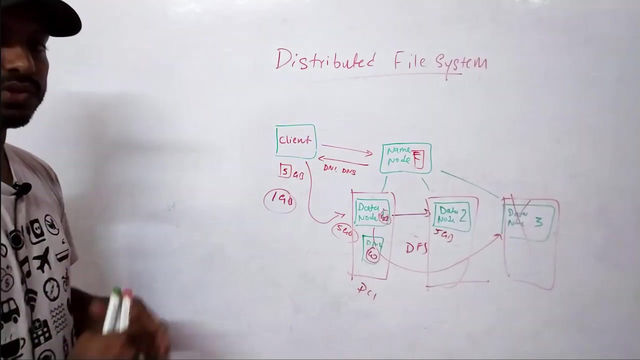 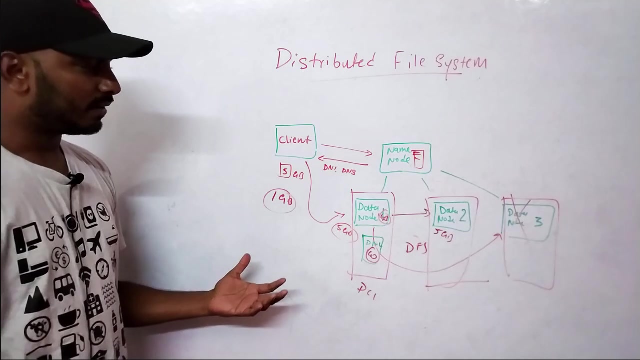 different location and different racks. so that way the data is still safe, um, and for the client it never feels like, okay, i, the data is somewhere, somewhere and it's very difficult to access. and it is a for for the client libraries. it will be so seamlessly accessible, just like how we access from a single machine. um, i think i have covered all of them. 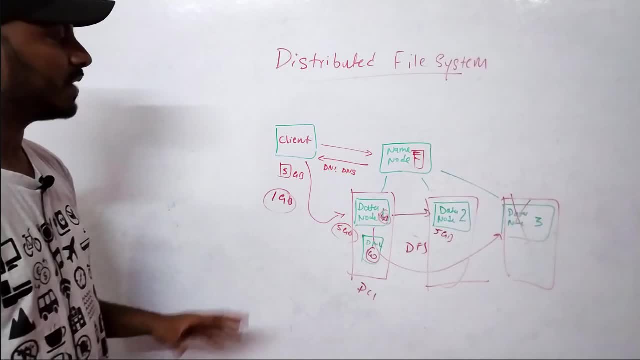 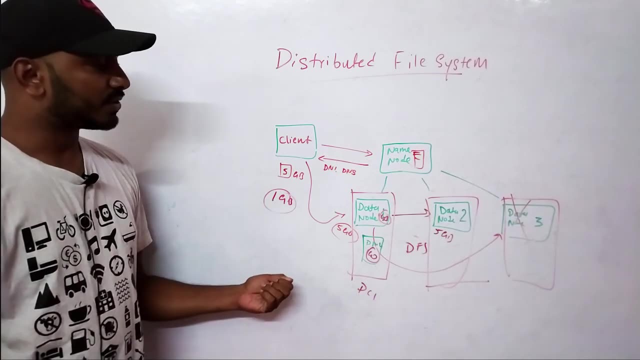 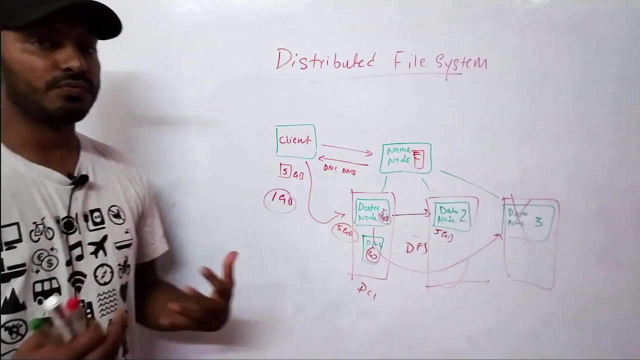 major information which you guys need to understand about the data file system. uh, think it like. it is just like any other file system which we use it in our machine machine, but the data is replicated across, you know, thousands of machines or if not hundreds of machines, but you, we don't even know how this data is. 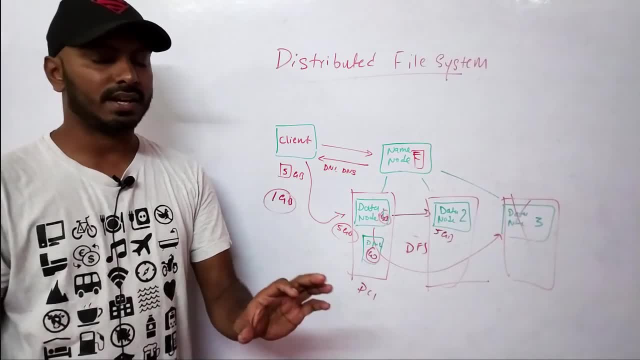 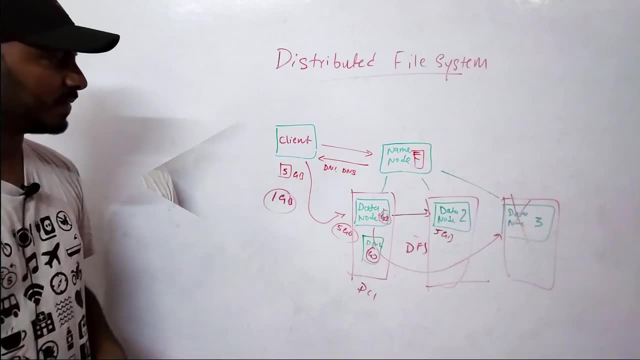 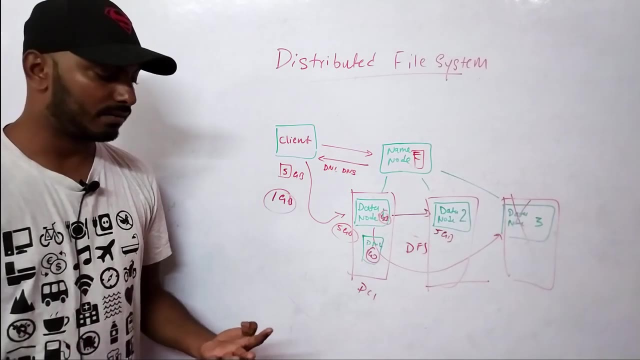 replicated and, you know, transferred between the data nodes. that's more likely. what you need to know about distributed file system and most of the technologies in Hadoop framework does support HDFS to read and write like spark. you know HBase. all of that technology is basically by default. 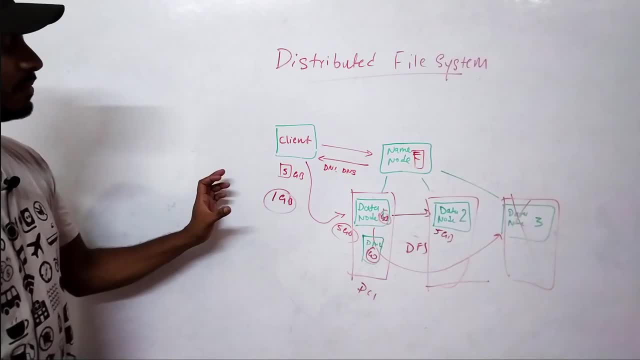 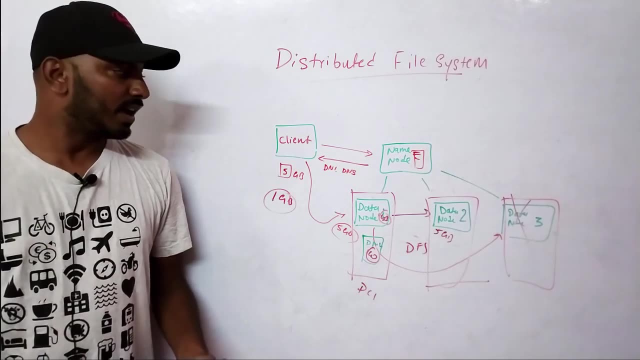 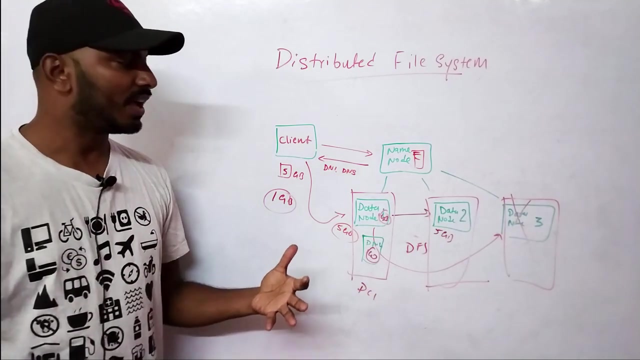 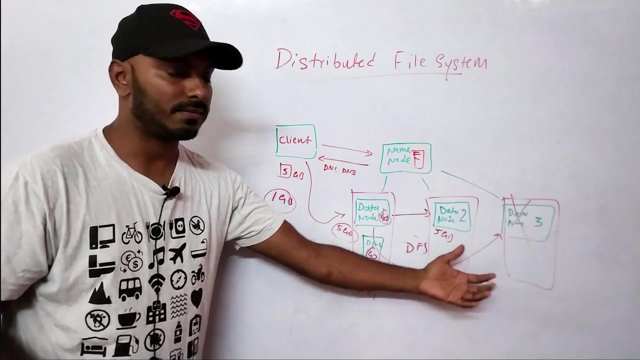 supports reading and writing it to HDFS based on some agreed protocols. so that's about the distributed file system. you can actually use the same pattern to design a lot of different. you know applications. maybe, wherever you want redundancy, wherever you want to keep the copy of data safely, you can basically use the same design of you having a name node and